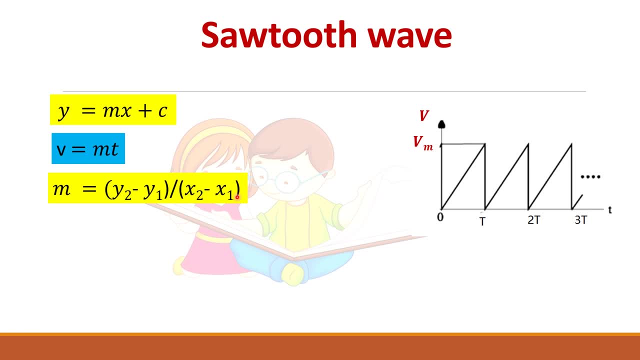 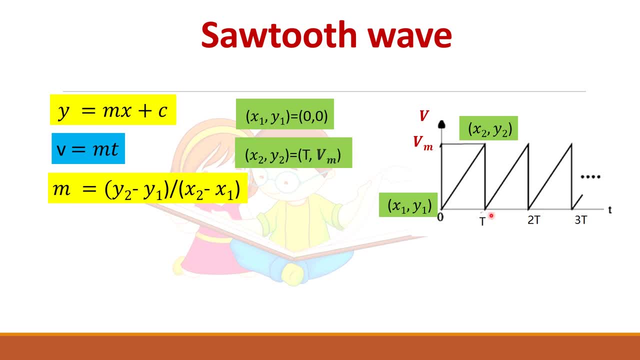 x variable, that is the horizontal variable, that is t, and for y2 we have vm. so t comma, vm. now let us substitute this here and find what is the slope. so slope is equal to vm by 2. so you can always remember this one easily, that whenever you are given a sawtooth waveform like this, whatever be, 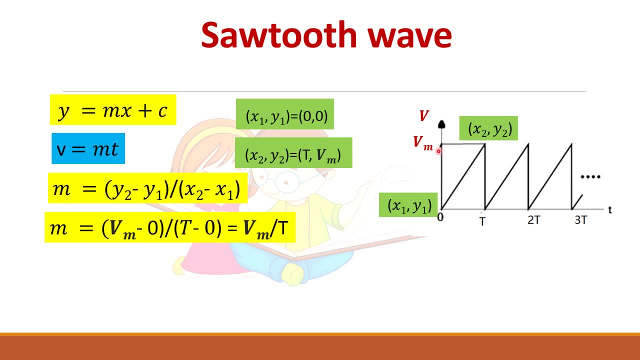 the magnitude given. you can simply write the slope, as this magnitude divided by t will be the slope of this line. now you substitute in this equation, v is equal to m instead of m. let us write the vm by t into t. so this is the equation we need to find. we need so that we can find the average value. 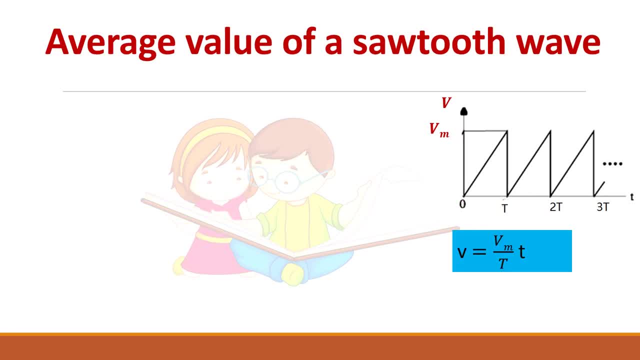 of the waveform. so now let us find the average value of this sawtooth waveform and the equation of the line we have found it. let us find the average value: v. average is 1 by time period: total time period t. integral of 0 to the same time period, t into. 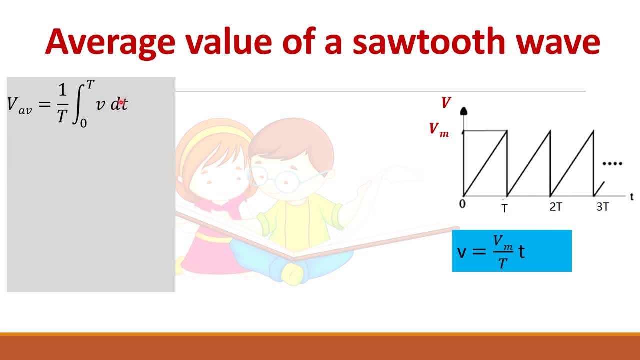 v into dt. see, here it is dt. so what is v? v is this equation? so now you substitute instead of v vm by t into t. here this is dt and t is here, so remaining two are constants, so we can take it outside. so it becomes vm by t square, integral of this small t alone. so if you integrate this t, it becomes t square by 2. 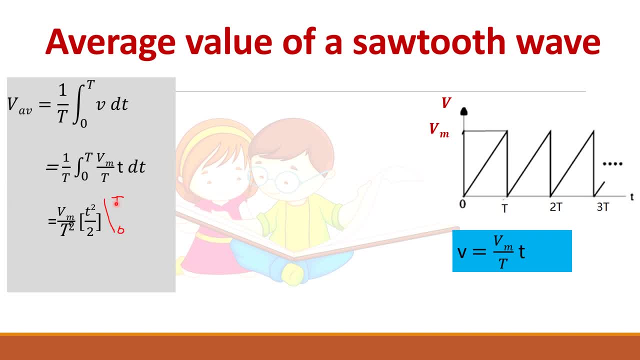 and now you apply the limits 0 to t so it becomes t square by 2. t square, t square get cancelled, so we can take it outside, so it becomes vm by t square, integral of this small t alone. so if you, your answer is vm by 2, so you can remember easily that whenever you get a triangular waveform or a 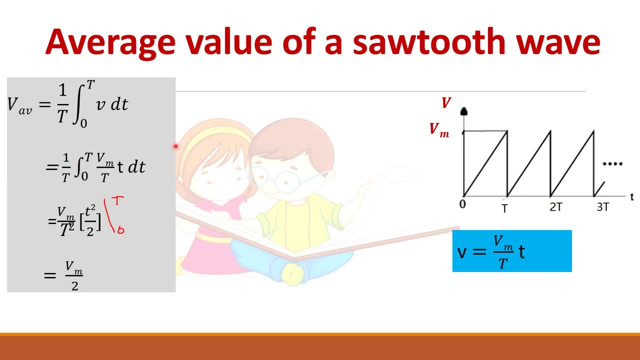 sawtooth waveform of this type. your average value is whatever is given here divided by 2. okay, so it is vm by 2. there is also another method where you can find the average value easily. so v average is equal to area under the curve, area under this curve divided by time period. so what is the area of this triangle? this? 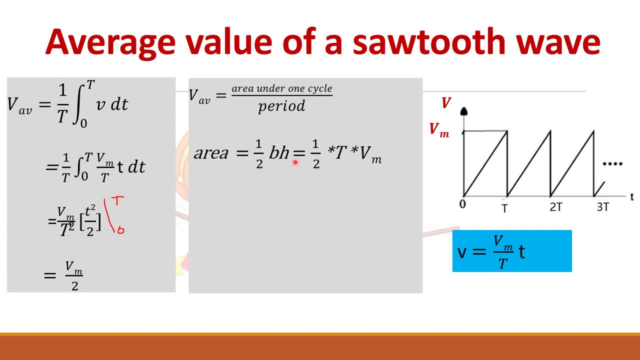 is a triangle, so area is half bh, half into base is t and height is vm. so this is the area divided by total time period is t. so what you will get again vm by 2, so you can follow any one method whichever is convenient for you, but the answer is: half of the magnitude will be your average value for this type. 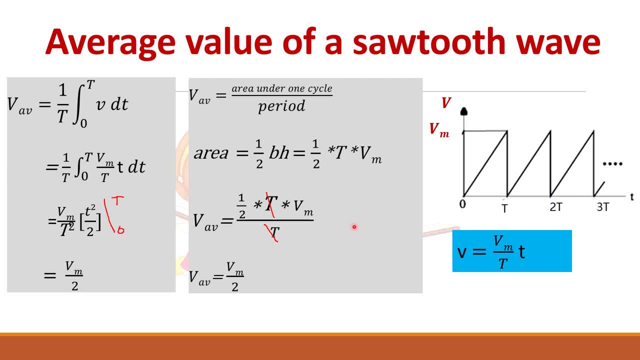 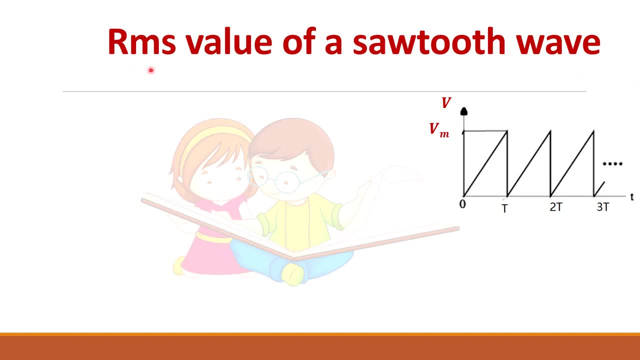 of waveform. now let us find the rms value of the sawtooth waveform. what you mean by rms root mean square. it means that first you have to square this waveform, then find the mean value of the sawtooth value, that is, average value, and then square root, that one that will be the rms value. so we know what. 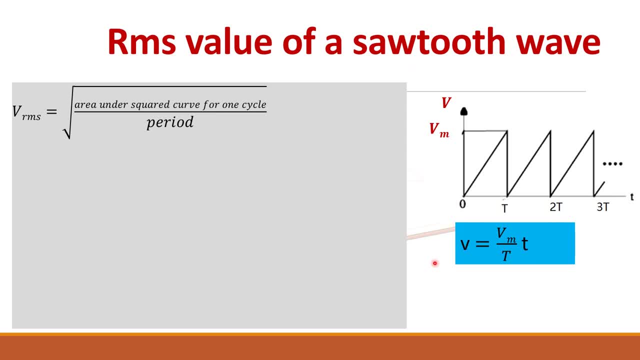 is v. so what is the squared waveform of this one? you square this one v square is equal to the whole thing you square it. so v? rms is equal to root of area under the squared curve divided by period. so let us see what is the rms value of the sawtooth waveform. so we know that this is the rms value of. 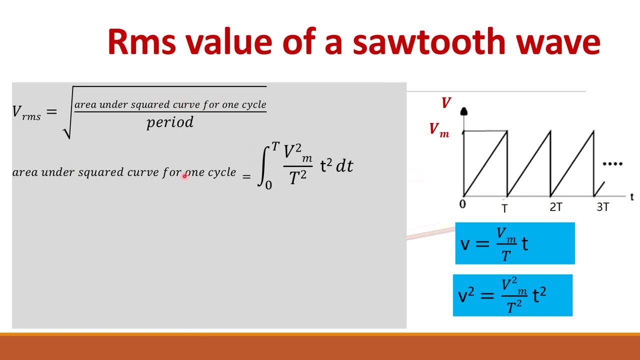 the sawtooth. so let us find the area under the squared curve first. so area under squared curve is equal to zero, to total time period divided by this waveform into dt. you put this equation here into dt, so let us integrate this one again. these two terms are constant. take it out and only. 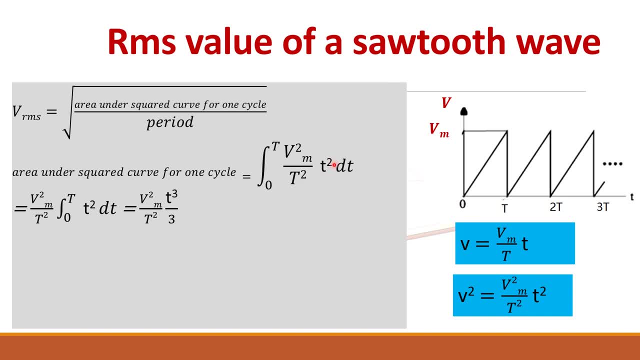 variable is t square. so if you integrate t square it becomes t 3 by 3. then you apply the limits 0 to t here and simplify it. you will get vm square t by 3. so v? rms is equal to this area divided by again one time period. so t gets cancelled. so you 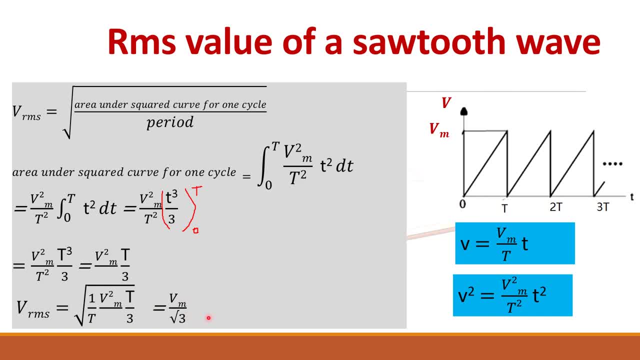 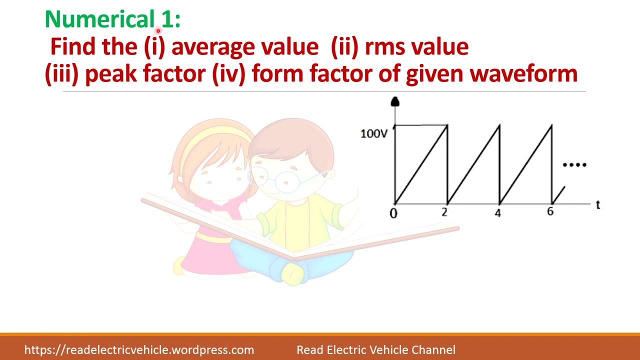 will get vm by root through root 3 as v rms value. so for a sawtooth waveform the rms value is vm by root 3, average value is vm by 2 and rms value is vm by root 3. now let us do one problem and find the values for the sawtooth waveform. so here vm is: 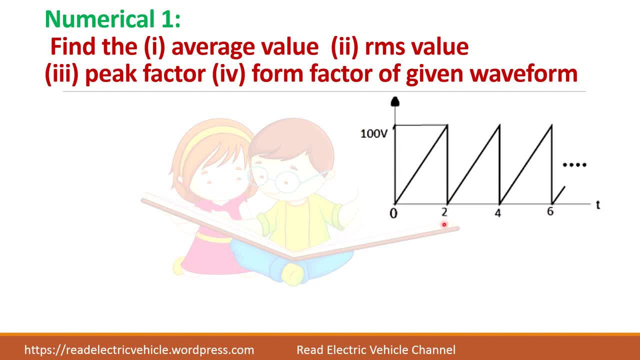 given as 100 volts and the time period is given as 2 seconds. so let us find the values for the sawtooth waveform so we will find out what is enough and we will only apply the average value. so these type of problems: normally you will get an objective type, so you will not. 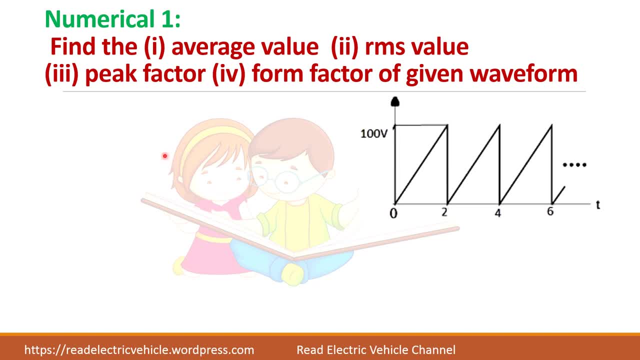 have time to write the formulas and calculate the value. you can directly apply the final equation and find it out the values. average value is equal to v. average is equal to vm by 2, so it is his 50 volts. rms value is equal to 3.8 times thisą. 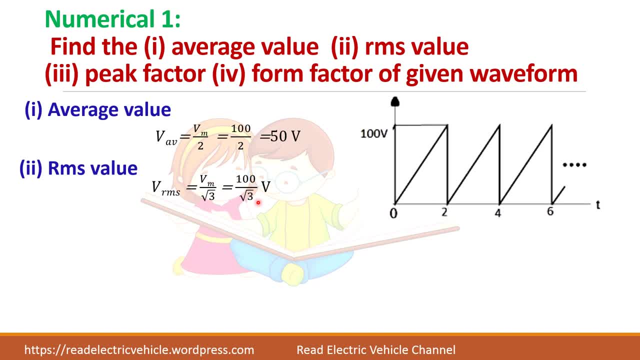 Vrms is Vm by root 3.. So you will get the answer. Then what is peak factor? Peak value divided by rms value is the peak factor. So what is the peak factor of any equation? That is the peak value. that is 100 volts here. So divided by this thing, So you will get root 3 and form factor is rms. 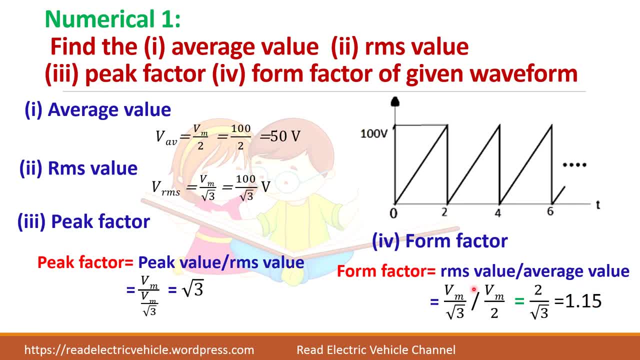 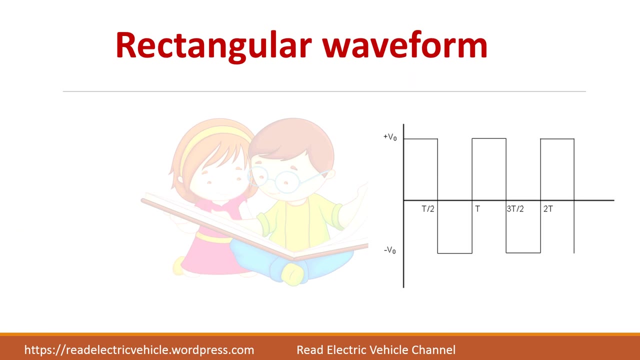 value divided by average value. So these things are direct calculation. you can do it. So when you get this type of problem in objective type or for two mark, directly write the formulas and you can find the answer easily. Now we have a rectangular waveform. that too, the waveform is symmetrical. 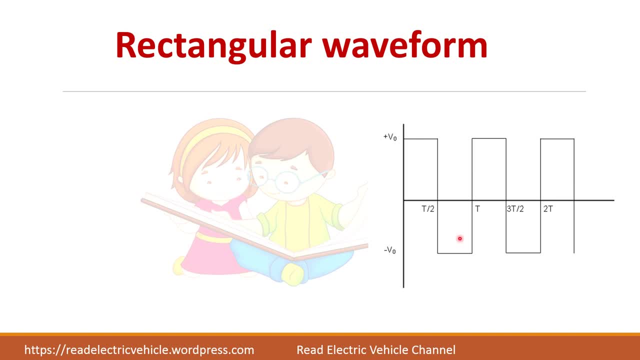 means that your positive half and negative half are same. So in that case you have to find the average value only for half cycle. If the waveform is symmetrical, always find the average value for half cycle. If you find it for full cycle you will get 0, because this half- positive half and negative half- will be equal. 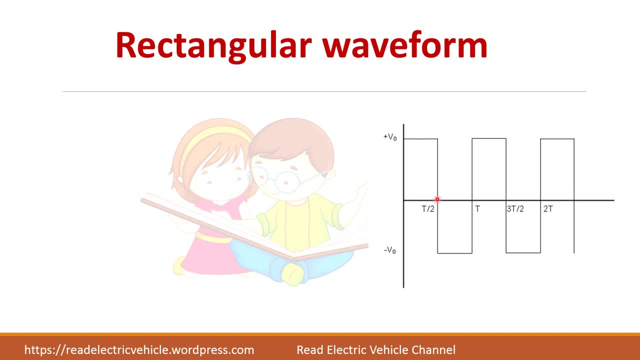 average will become 0. So always try to find the average value only for 0.. Half cycle, So you can find v average is equal to area under the curve divided by time period. Time period: you take it as t by 2. So area of rectangle is base into height. So v average will be equal to. 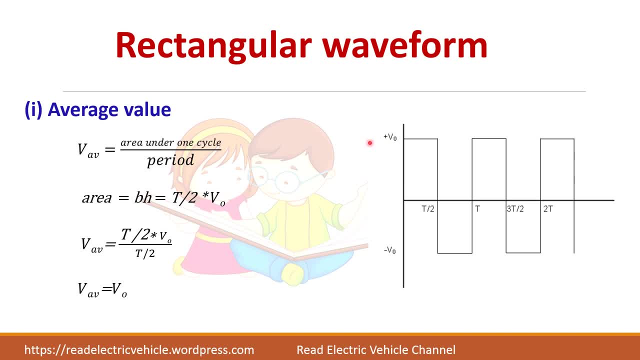 v naught. So regardless of the magnitude you can blindly write, v average is equal to whatever value it is given, Suppose it is given as t by 2. So you can find v average is equal to v naught. And this пример you can divide by the number of. if you calculate that you are lower than 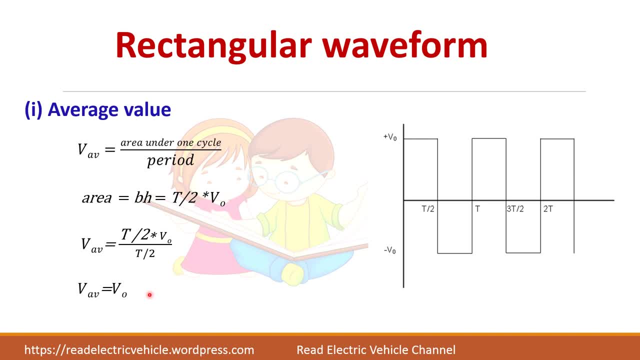 0 curve, you get 0. that is still v. average is equal to 100.. If you can find han flag, is that a number, So you will get happiness. okay, That is which has a Which where v is the amcent Ok. 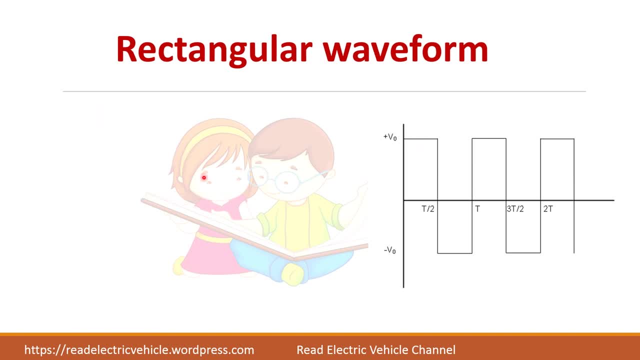 For a rectangular waveform it is very easy to find the average value. that will be equal to the maximum value. Now let us find RMS value. So RMS value. square root of area under squared curve divided by period, So area under the squared, so it is b naught. square root of area under squared curve divided by period, So area under the squared, so it is b naught. squared to the area under squared, So it 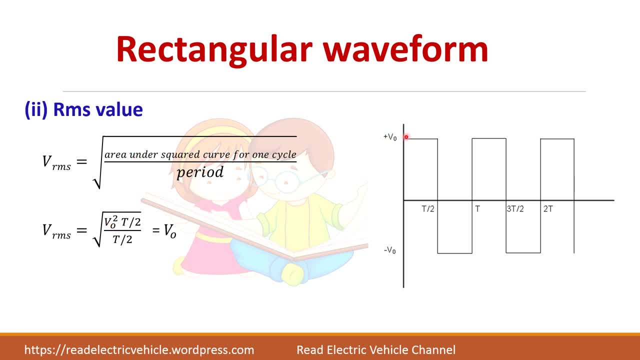 So area of the square. so it is B naught square into time period t by 2 divided by t by 2.. So that again comes to B naught. It means that for a rectangular waveform average value and RMS value, both are equal to the maximum peak value. 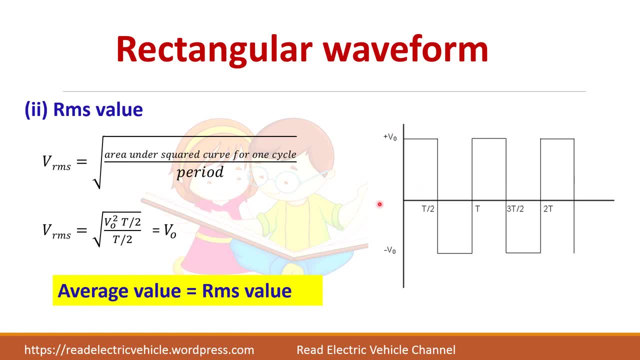 So rectangular waveform is the easiest to find. the average value and RMS value. Remember, all these things are applicable, only the waveform is symmetrical. Sometimes they will give here some 100 volts and here minus 200 volts. At that time this formula will not satisfy. 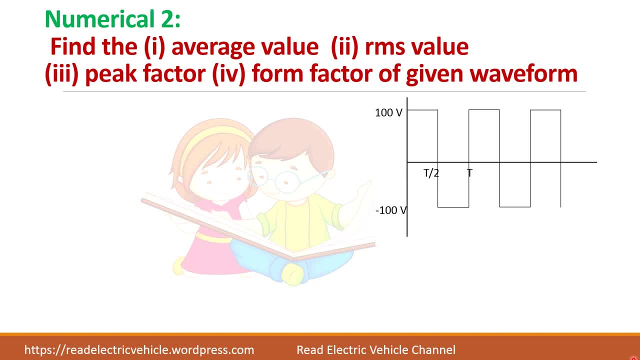 Now let us Do one problem and find the average value, RMS value, peak factor and form factor for the waveform. So see here: it is given as 100 volts and minus 100 volts, So the average value is equal to 100 volts. 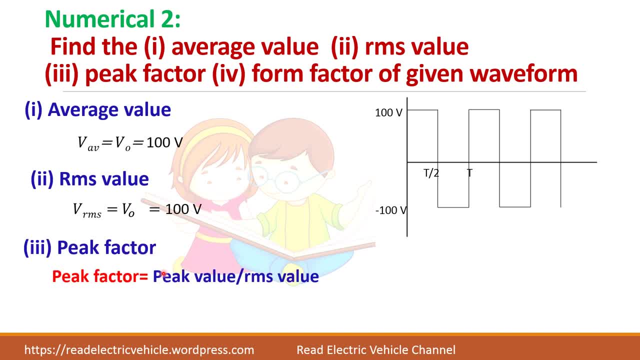 RMS value, also 100 volts. Peak factor is peak value by RMS value. So peak value is also 100.. RMS is also 100.. So peak factor is 1.. Form factor: RMS. by average. again it is also equal to 1.. 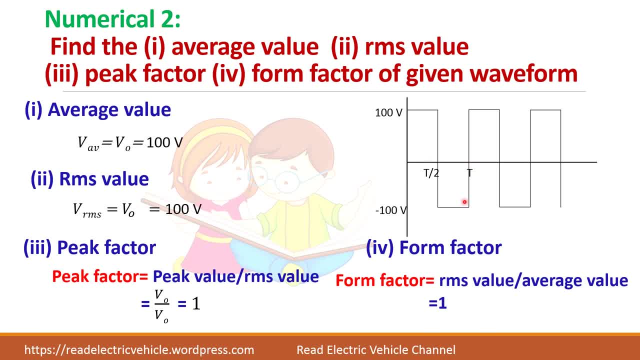 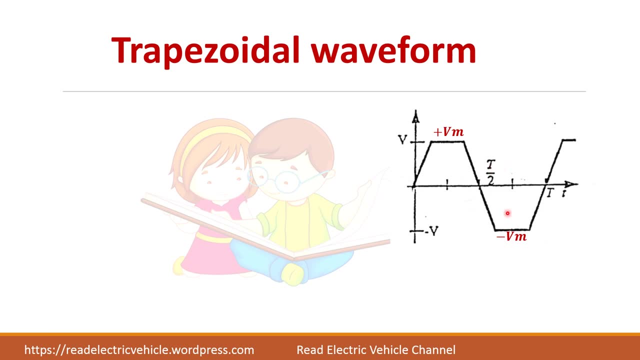 So if you are given this type of problem in objective type, don't skip the question. It is very easy to remember the formula. Next, we have a trapezoidal waveform. This waveform is also symmetrical, with magnitude of plus Vm and minus Vm, and the total time period is t. 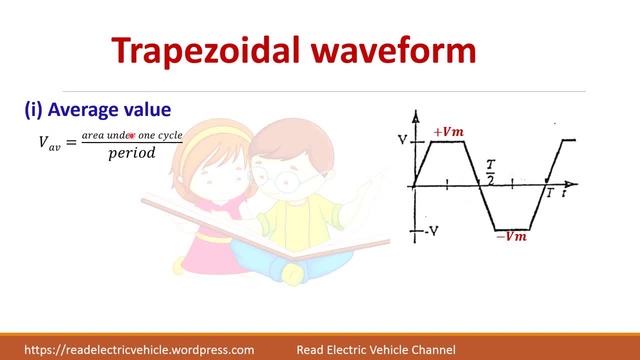 So Let us find the average value That is given by area, total area divided by time period. So what is the area of the trapezoidal waveform? You see this one. It actually consists of three parts: Here one triangle, here one triangle, and in between you have a rectangle. 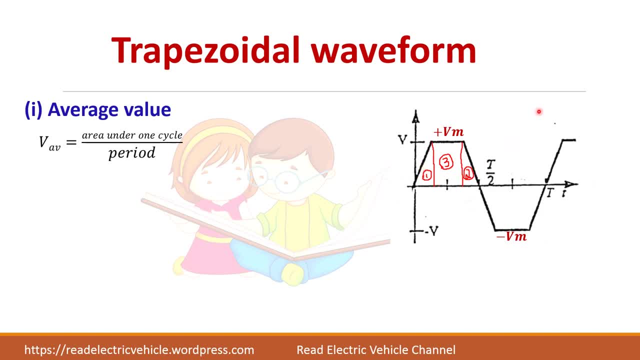 So if you split it like this, it is easy to find the area. So you know the area of a triangle that is half BH. So you know the area of a triangle that is half BH. So let us mark the time period first. 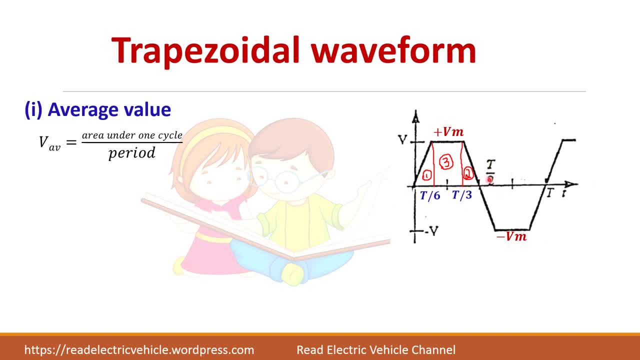 So the total time period for half cycle is t by 2.. So divide by 3.. So it becomes t by 6.. Here it is t by 3.. Okay, So now area of the triangle is equal to half into BH, half into base. 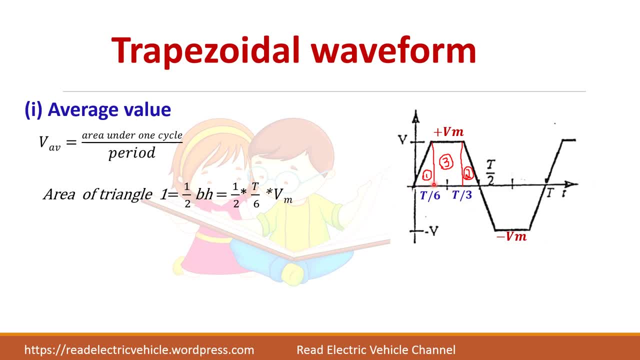 What is the base? T by 6 is the base of this first triangle. Okay, So what is the base? It is t by 6 into height. Height is BM, So you get this area the same magnitude. you will get for this triangle too, also. 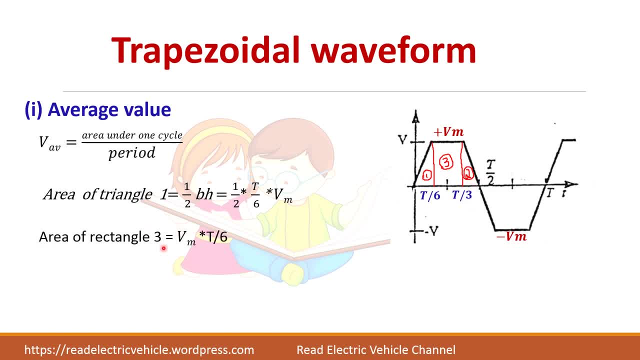 So area of the rectangle is base into height. What is the base? This time period is again t by 6 into magnitude BM. So you add all the three areas: triangle one, triangle two, plus this rectangle. You add all the three areas, So this is the total area. So it comes around. 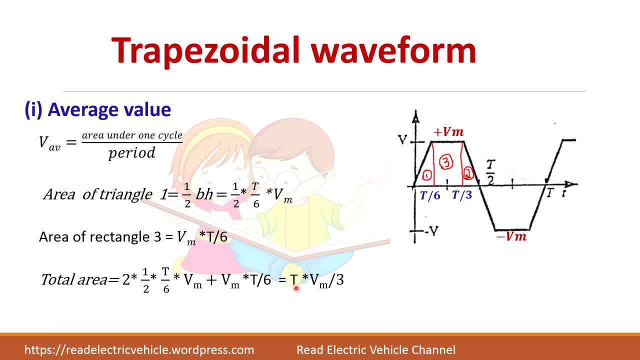 Vm by 3 into time period. So this is the total area. So V average is equal to this area divided by time period, t by 2.. So you will get 2 Vm by 3 as the average value for the trapezoidal waveform. 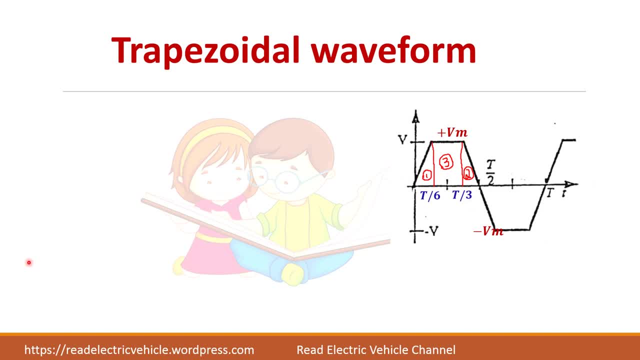 Now let us find the RMS value for the trapezoidal waveform V. RMS is area under the squared curve, So you have to find the area of the squared curve. So what is the area of the squared triangle? Already we have done this derivation in sawtooth waveform. 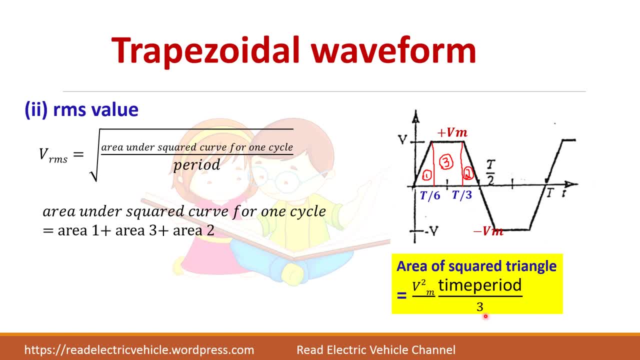 Same thing. So Vm square into time period divided by 3.. So area this, area 1 and the area 2 will be same thing: Vm square into time period divided by 3.. So what is that Vm square into? what is the time period? 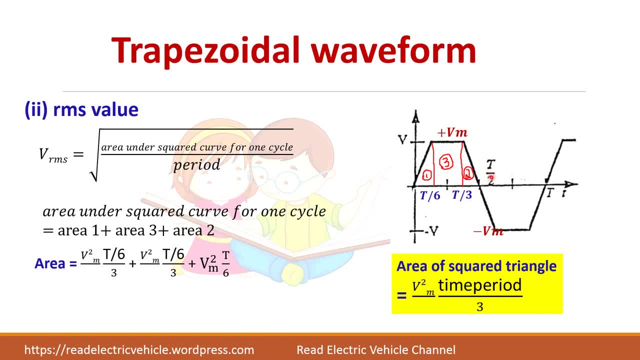 You see, for half cycle total time period is t by 2. So you divide into, because you have three portions here. So divide this by 3. You will get t by 6.. So t by 6. This is t by 3, and this is total time period is t by 2.. 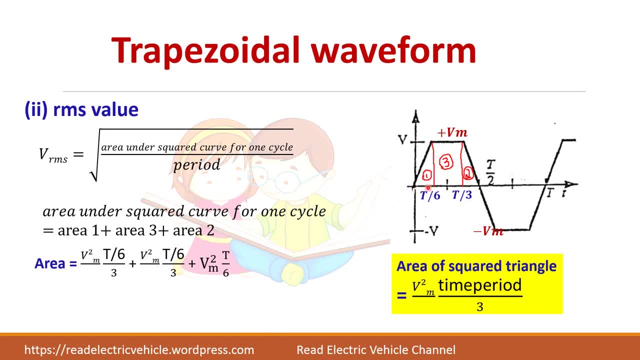 So Vm square into time period for this triangle is t by 6 divided by 3.. Again for this part also same thing, And for rectangle the area is base into height. So here you have to square that magnitude. Vm square into time period is t by 6.. 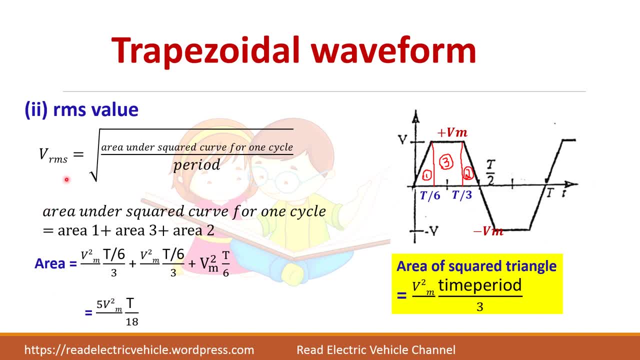 So area, you got the area. Now again, you have to find what is Vrms. Vrms is equal to area divided by time period. So area is this: one divided by time period, t by 2.. So find the square root of that. you will get the Rms value. 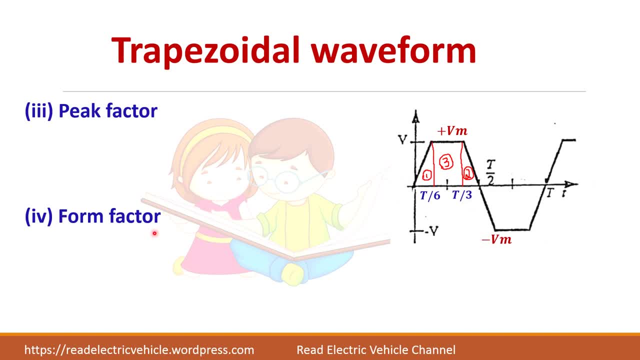 Next we will find what is peak factor and form factor Already. we know the formula: peak value is Vm substituted and form factor, you will get 1.118.. So we are able to find the Average Rms value for the trapezoidal waveform easily by splitting into three parts. 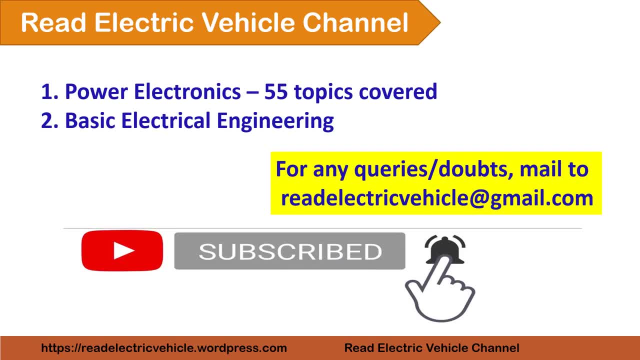 In this channel. already 55 topics have been covered in power electronics subject And most of the topics are covered in basic electrical engineering. If you need any other topic, just mention in the comment section. If you have any doubts in the video, you can mail to this email id. 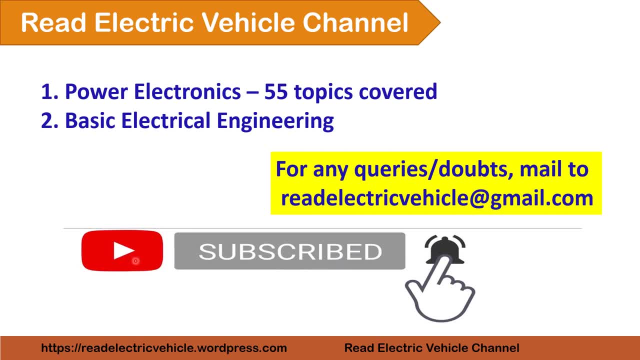 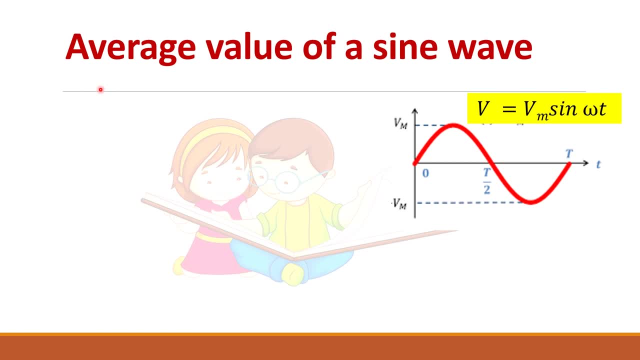 And if you like the video, please do subscribe to this channel. Thank you. Now let us see the average value of a sine wave. As we know, the instantaneous value of a sine wave is: V is equal to Vm. sine omega t, Apply the formula. 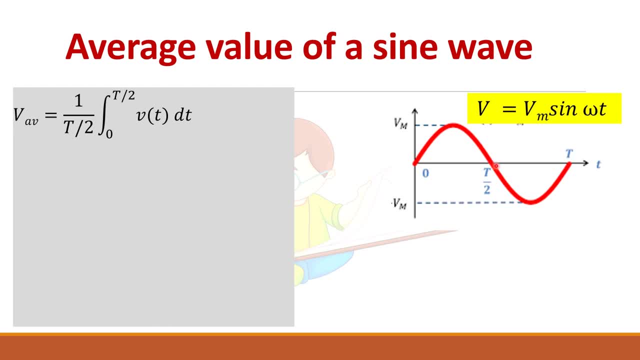 So it is a symmetrical waveform. So let us take half cycle. So the time period is t by 2.. Integral of 0. 0 to t by 2 into V of t. What is V, Vm sine omega, t? 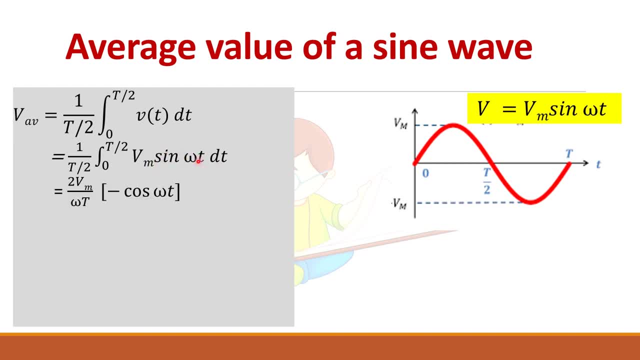 So integrate this one. So integral of sine omega is minus cos omega t divided by omega. Since you have only dt here, When you integrate this one, you will get one omega term, which have taken this side. So apply the limits. 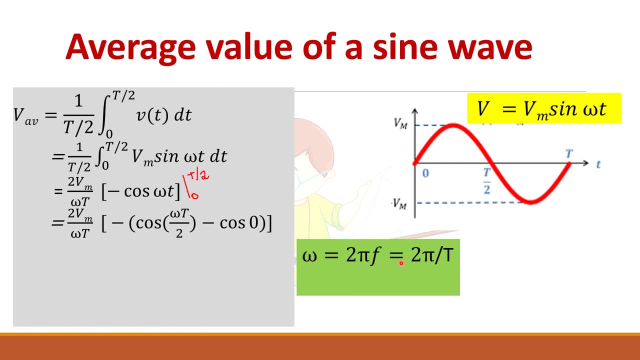 And omega is 2 pi. f Means that f can be f is 1 by t, So 2 pi by t. So omega t is equal to 2 pi. Simplify this one So you will get 2 Vm by pi as the average value of a sine wave. 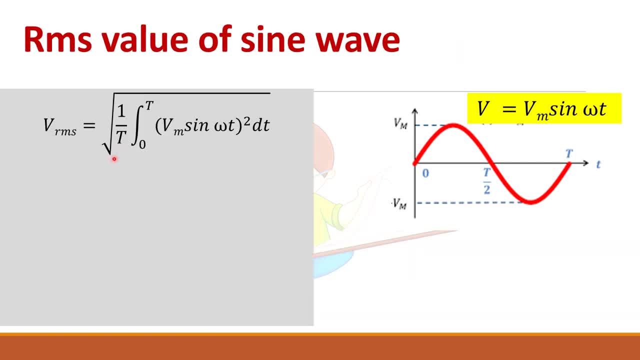 Next we are going to find the RMS value of the sine waveform, So 1 by t, integral of 0 to t. You have to find the Square waveform, So Vm sine omega t, The whole square, That is this V square. 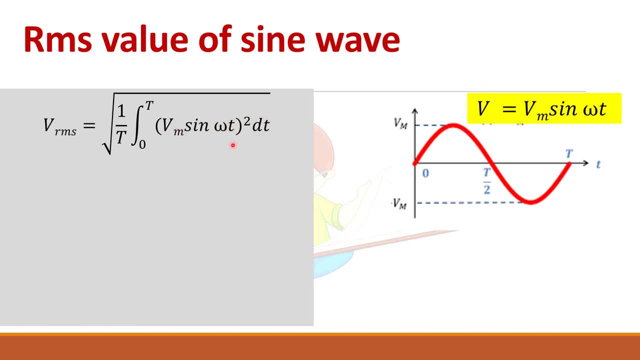 Means you square it into dt. So sine square We cannot do integration. So simplify this one into 1 minus cos 2 omega t divided by 2.. So this is a direct formula. Apply it. Take this 2 outside. 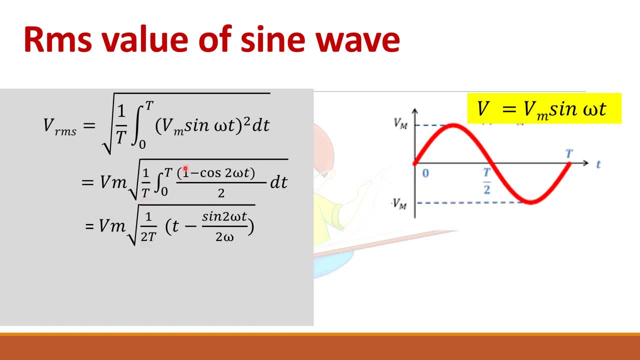 So it becomes 2 t. Now you integrate this one, so 1 becomes t and cos 2 omega t. if you integrate, you will get sin 2 omega t divided by 2 omega. now you apply the limits 0 to t. simplify it: what is omega t? it is equal to 2 pi. 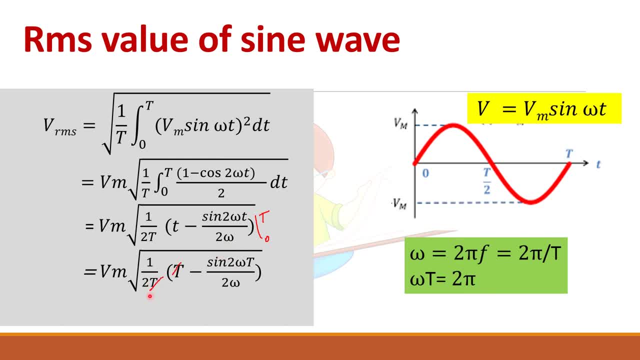 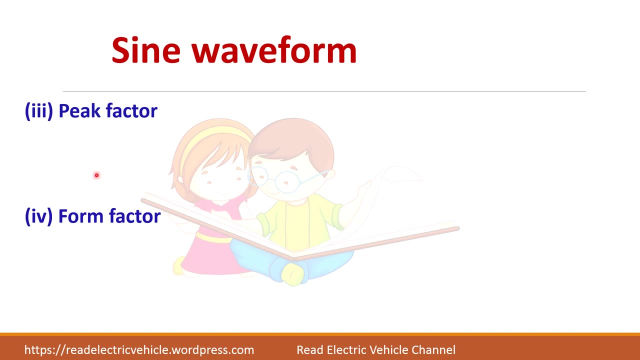 so you substitute here this becomes 0, so you get cancelled. so your answer is vm by root 2, so v? rms is equal to vm by root 2. next we will find the peak factor and form factor, so which is a direct formula, substitute the values, you will get peak factor as 1.414. 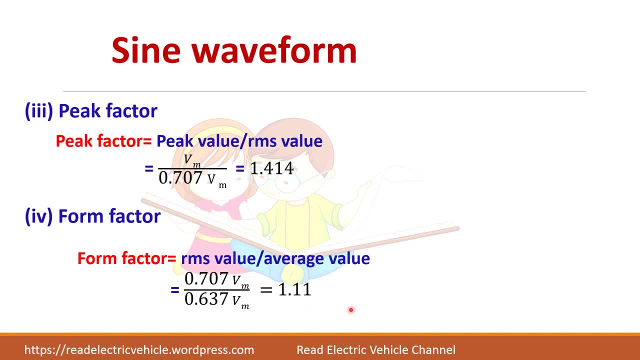 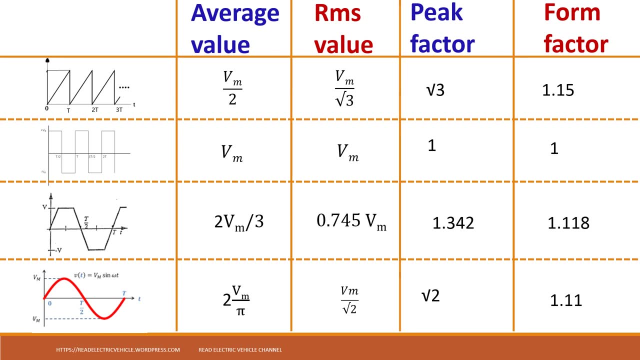 and form factor is 1.11. now this is a table which summarizes what we have learned in this video. we have taken four different waveforms and we found the four important factors for each of the waveform and i have summarized here so you can see that: for rectangle, it is easy, vm, vm. 1, 1, okay, it is very easy. and for sine: 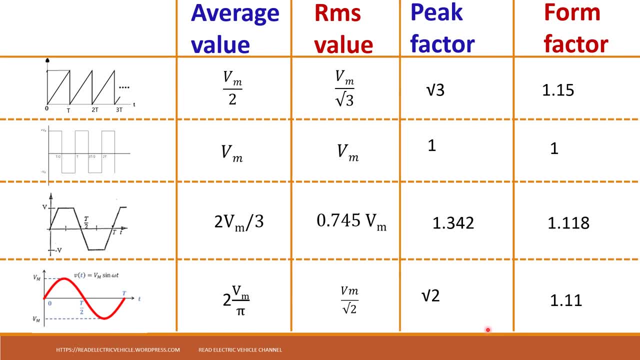 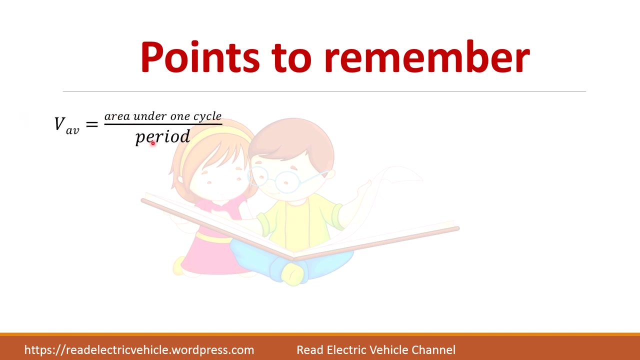 waveform you remember because it will be used in most of the problems you will be given about sine waveform. so 2 vm by pi is the average value and rms value is vm by root 2. so the points to remember here are: average value formula is area under the curve divided by